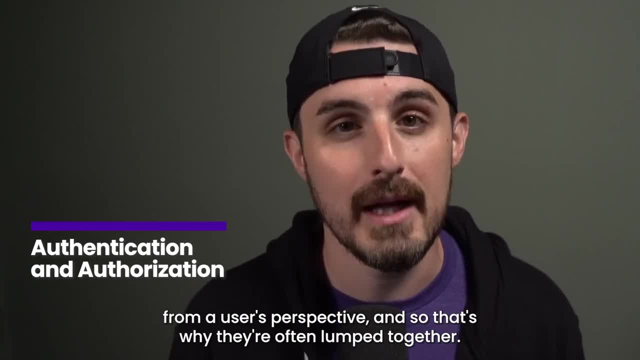 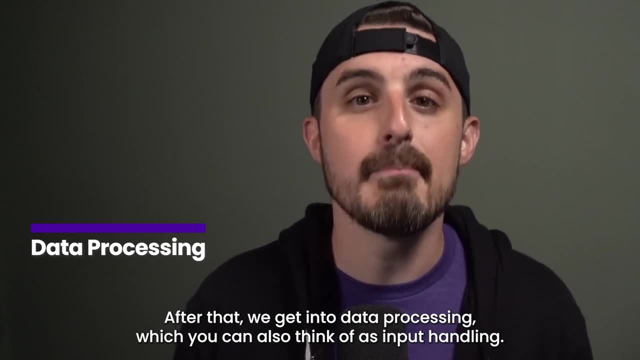 These two things tend to happen simultaneously from a user's perspective, And so that's why they're often lumped together. After that, we get into data processing, which you can also think of as input handling Need to make sure that, when users are providing data into your system, 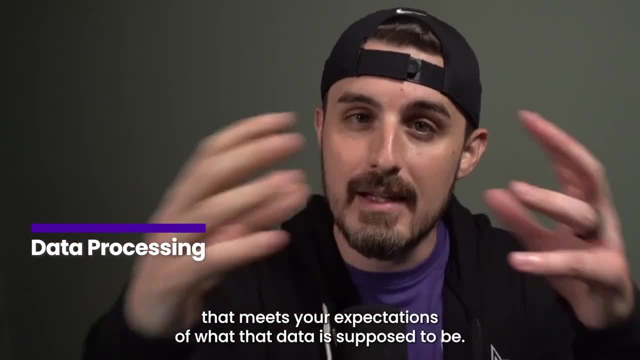 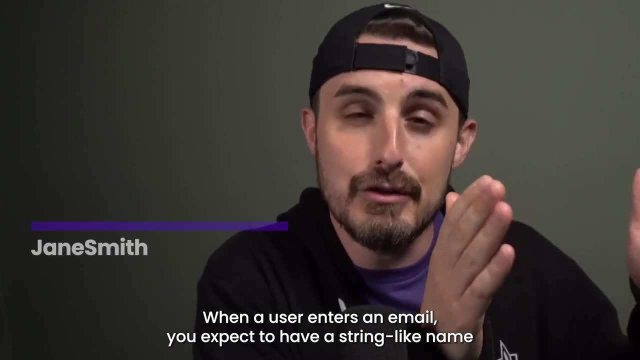 they do so in a way that meets your expectations of what that data is going to look like. As an example to illustrate this, think of an email. When a user enters an email, you expect it to have a string like name, an et symbol, and then a domain like googlecom or gmailcom. 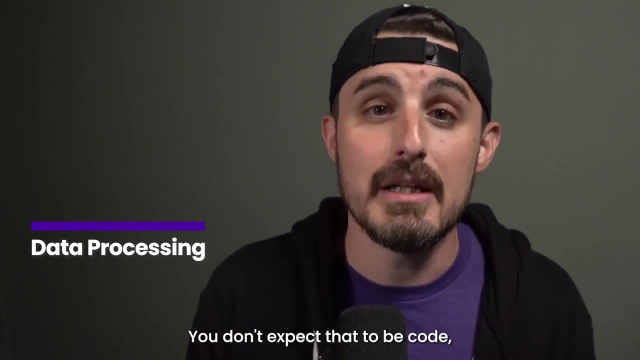 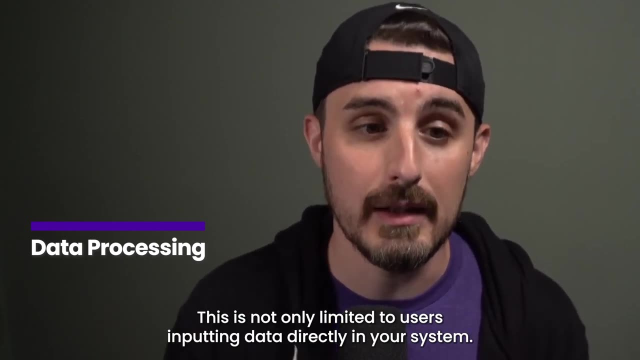 But you don't expect that to be something else, You don't expect that to be code, And you need to make sure that somebody isn't trying to do that within that field. This is not only limited to users inputting data directly in your system. 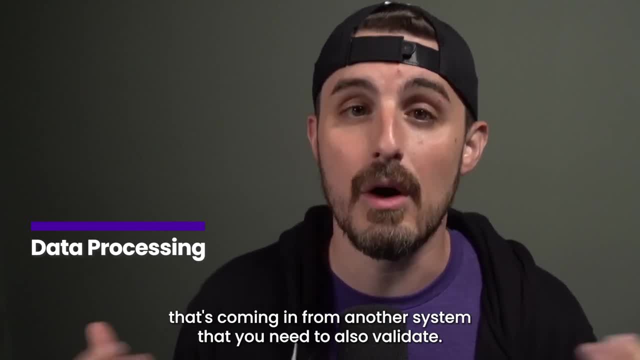 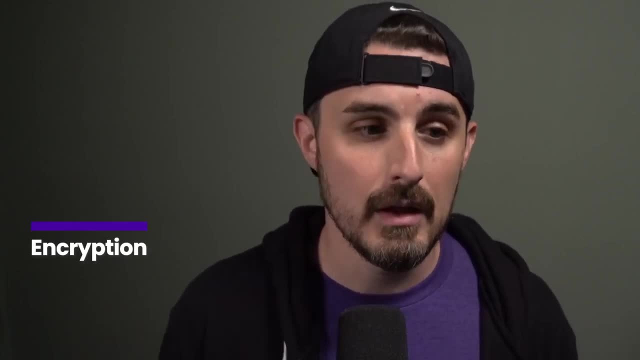 This could be data that's coming in from another system that you need to also validate. Think of them as like APIs And so forth. Next up, we have encryption, which can mean a lot of things- The simplest way I would describe it, and I might be oversimplifying things here. 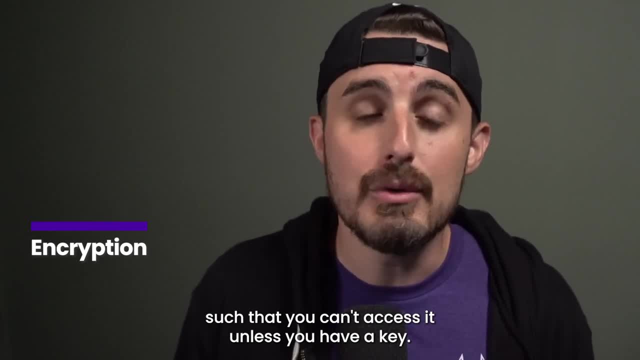 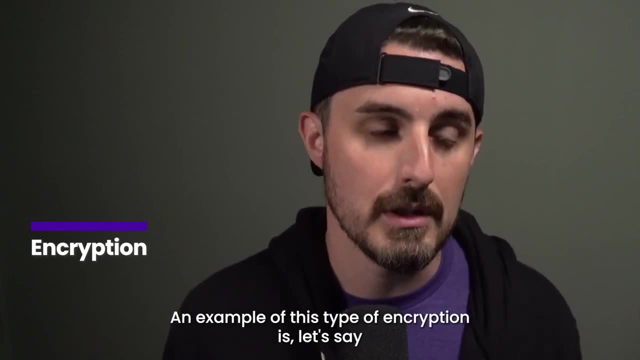 but it's about sealing and locking information such that you can't access it unless you have a key. So even if someone steals the data, they can't really do anything with it without the key. An example of this type of encryption is: let's say, you have data inside of a database and you want that data to be encrypted. 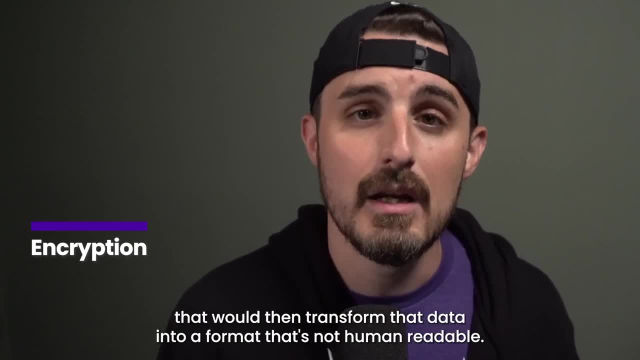 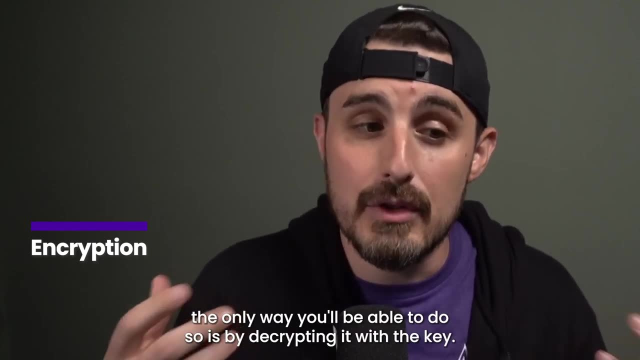 You would use an encryption algorithm along with a specific key that would then transform that data into a form And that's not human readable, Then, in order to access that data, the only way you'll be able to do so is by decrypting it with the key. 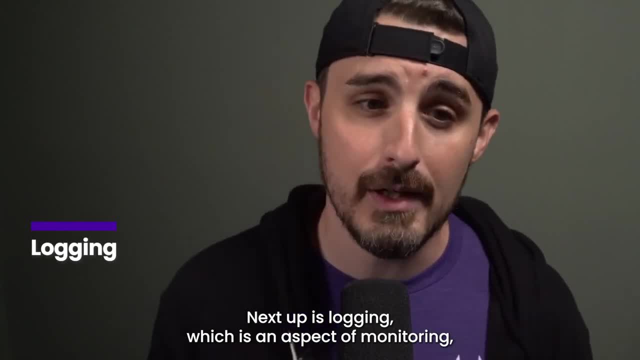 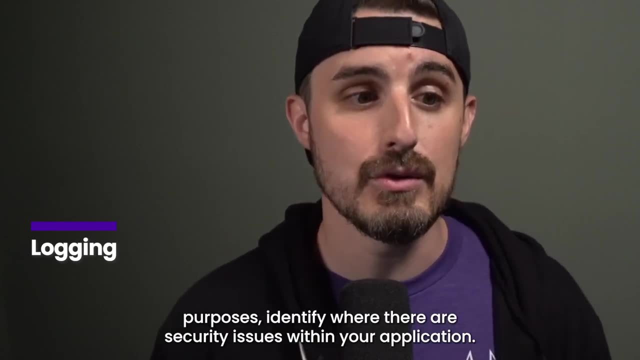 All right. Next up is logging, which is an aspect of monitoring And, if you're fancy, observability. Logging is a way to help detect and, for research purposes, identify where there are security issues within your application, For example, logging information about what a user might be doing. 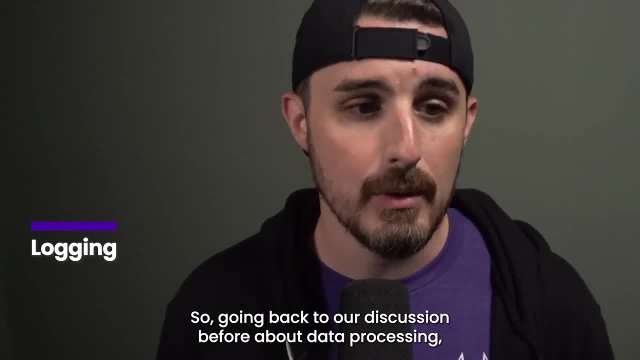 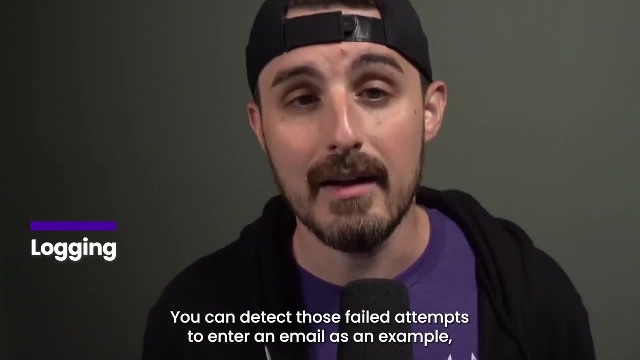 or attempting to do that's malicious in your app. So, going back to our discussion before about data processing, when somebody is trying to input malicious data in an email field, let's say you can log that. You can detect those failed attempts to enter an email as an example. 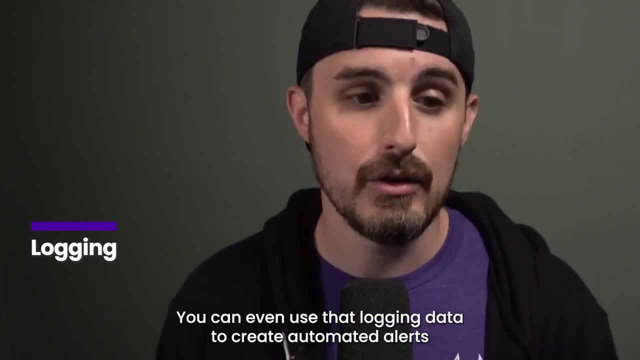 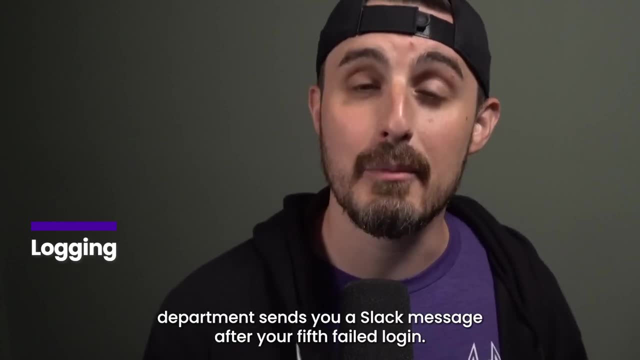 which will help in identifying and blocking bad actors. You can even use that logging data to create automated alerts based on certain thresholds, Like when your IT department sends you a Slack message after your fifth failed login. And last but not least, is testing Now typically to developers. testing consists of: 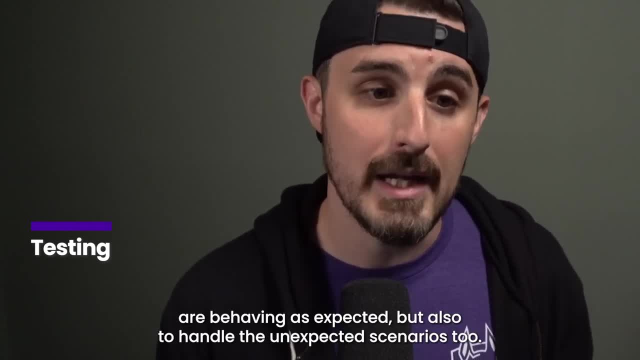 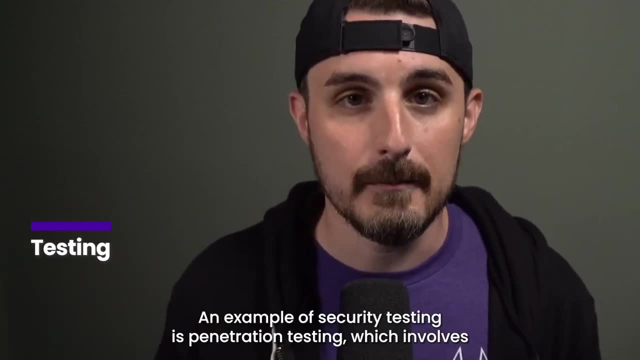 ensuring the functions and operations within your code are behaving as expected, but also to handle the unexpected scenarios too. But that's just one area of testing. In addition to that, there's security testing. An example of security testing is penetration testing, which involves having security researchers and experts. 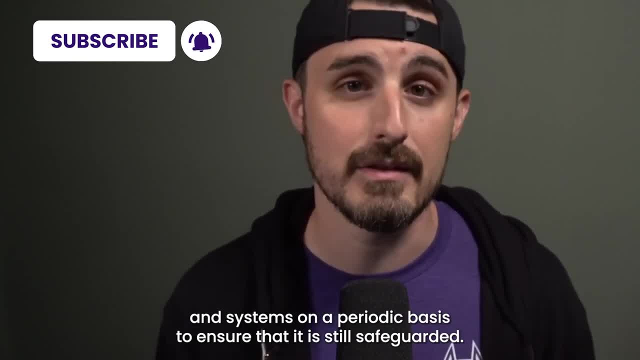 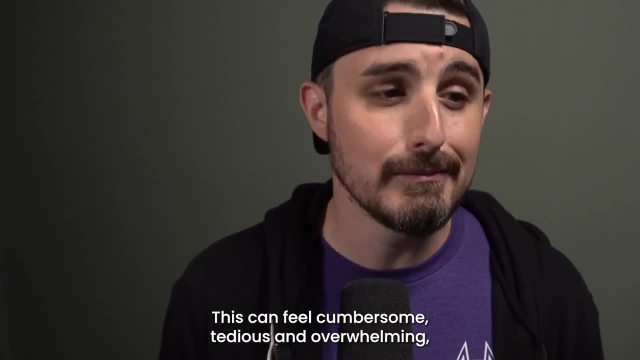 attempt to break into your applications and systems on a periodic basis to ensure that it is still safeguarded, And that is a brief overview of how we can secure applications. This can feel cumbersome, tedious and overwhelming, especially if we're doing this manually. 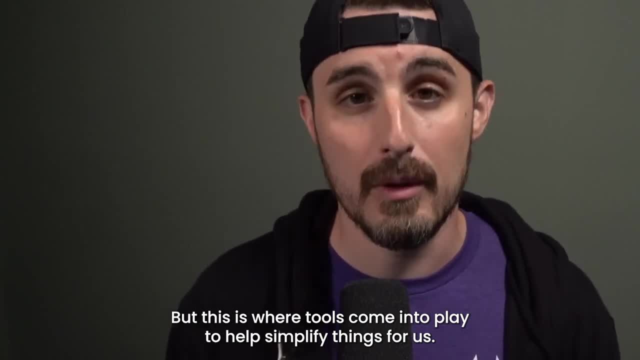 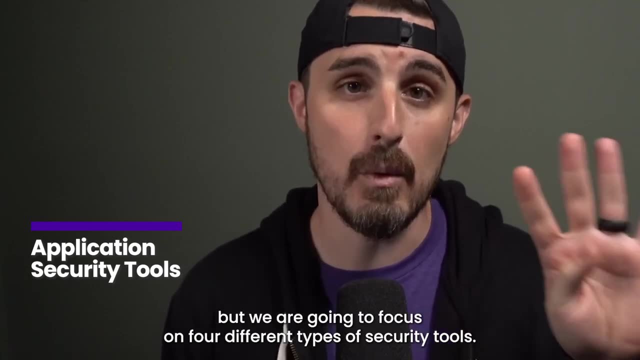 But this is where tools come into play to help simplify things for us. What are some tools that can help us secure our applications? Well, there are many out there, But we are going to focus on four different types of security tools, That is, software composition analysis, static application security testing. 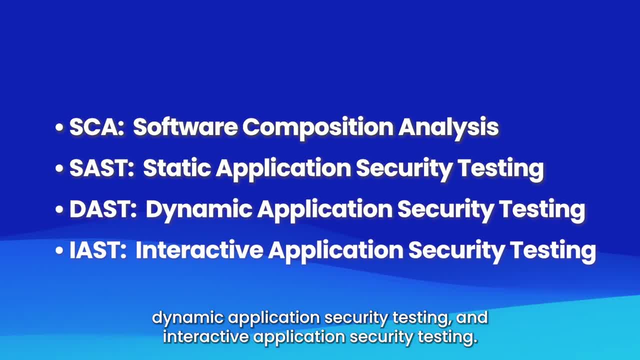 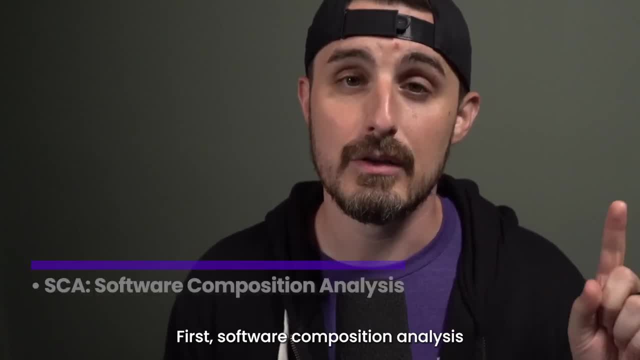 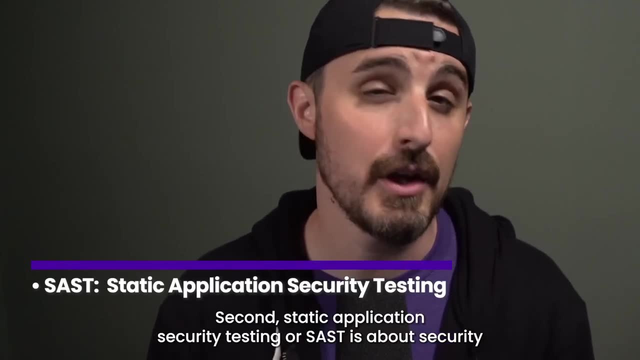 dynamic application security testing and interactive application security testing. Now I'm going to dive into these deeper, but here's the quick summary of them. First, software composition analysis, or SCA, is about security scanning of your dependencies. Second, static application security testing, or SAST. 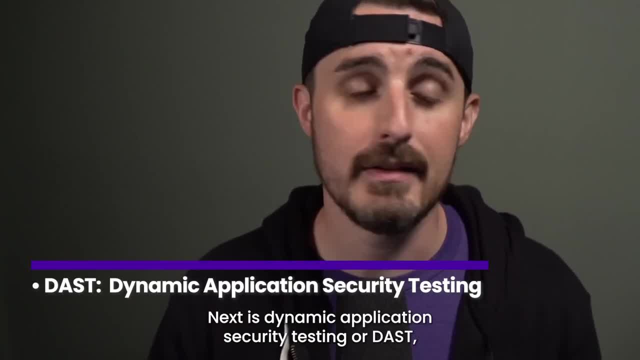 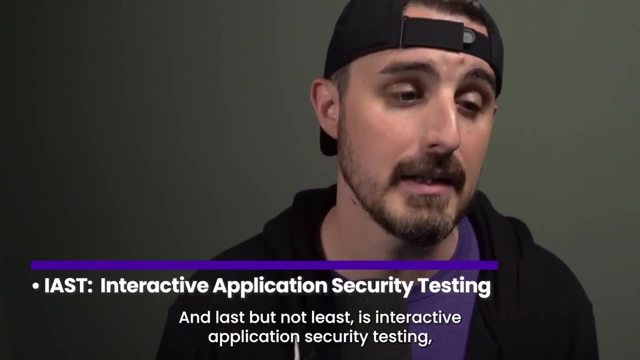 is about security scanning of the code you write. Next is dynamic application security testing, or DAST, which is about scanning your code while it's running. And last but not least, is interactive application security testing, which is about scanning your code while it's running and users are using it. 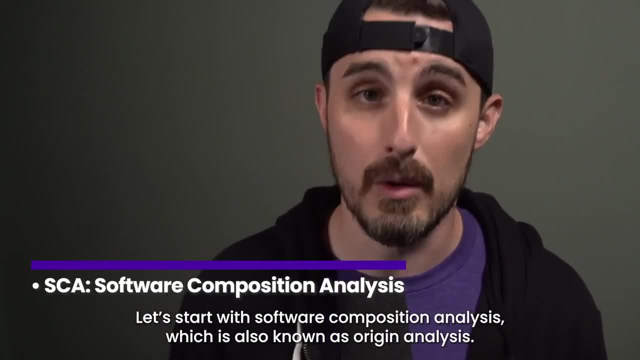 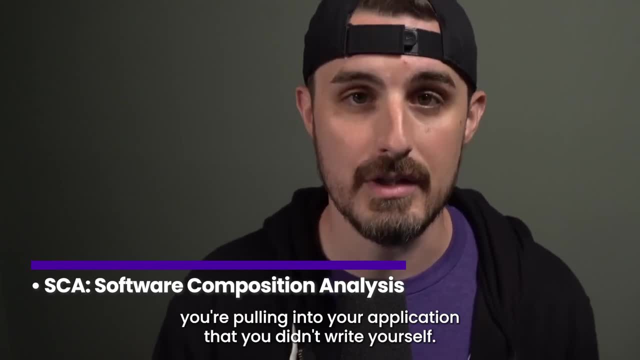 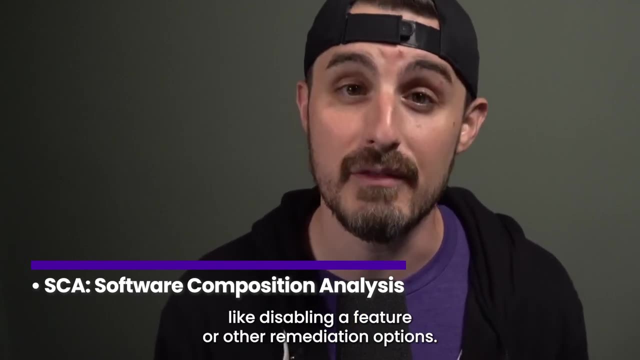 Let's start with software composition analysis, which is also known as origin analysis. This method analyzes all the software components and libraries you're pulling into your application that you didn't write yourself. SCA tools help you identify known vulnerabilities and notify you of any patches, config fixes like disabling a feature, or other remediation options. 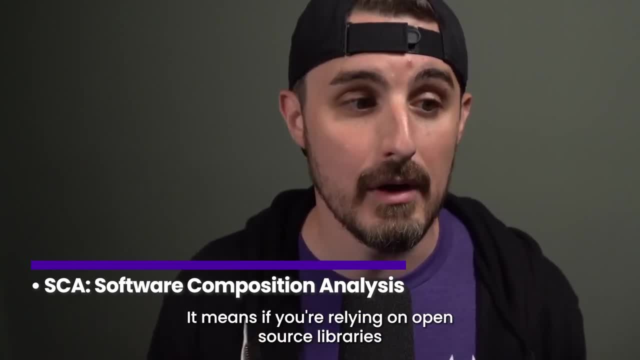 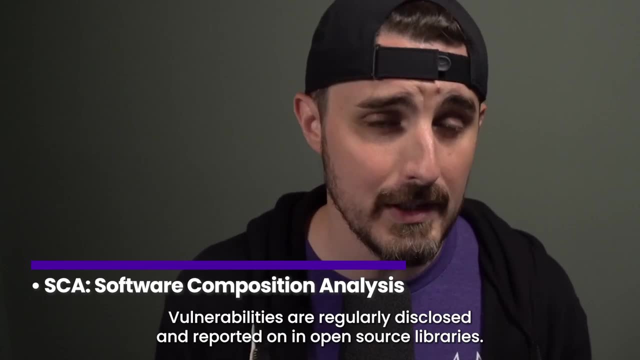 What does that mean in practical terms? It means if you're relying on open source libraries that you pull into your application, you need a SCA tool to actively monitor those libraries for vulnerabilities so you don't have to. Vulnerabilities are regularly disclosed and reported on in open source libraries.